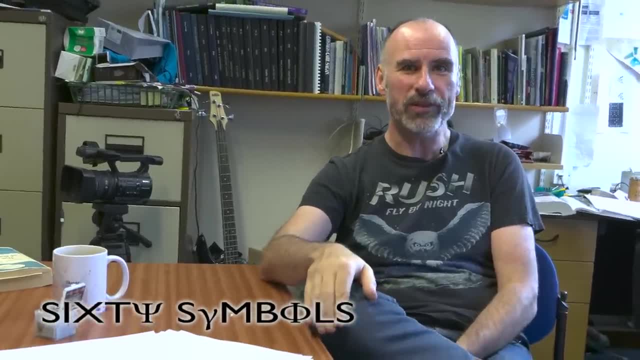 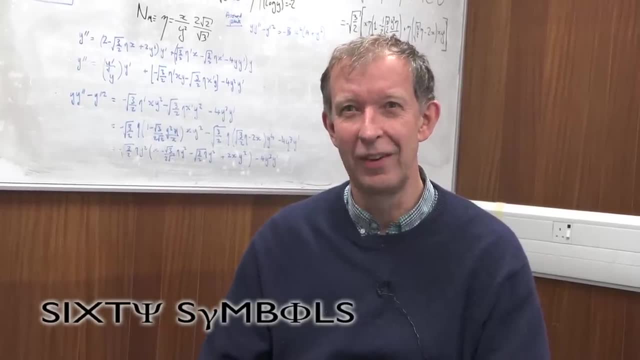 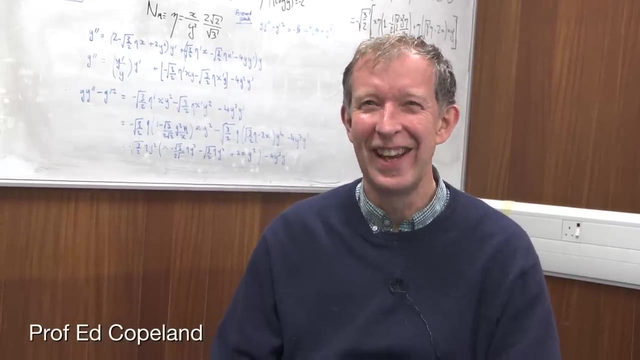 I'm absolutely delighted. It is about bloody time that the people who won the Nobel Prize won it. When I was a student, you were told: don't go there, Do not go into the foundational aspects of quantum mechanics. What does it mean? What does an observation mean? And just calculate? 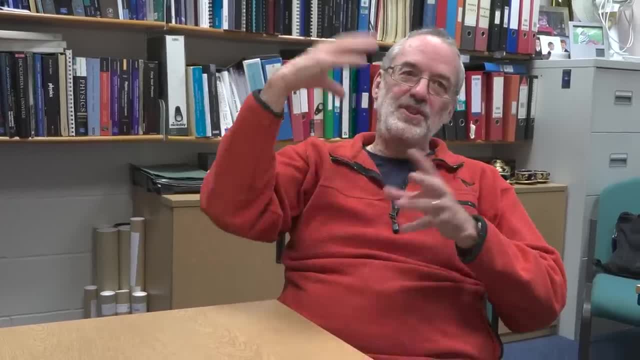 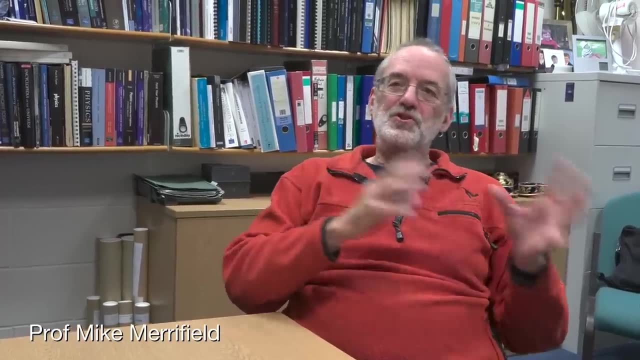 because it works so well. This is talking about weird quantum states. I mean this weird quantum state when it comes to Nobel Prizes. On the one hand, they kind of irritate me a bit because they oversimplify. You know, there were masses of people involved in this work. There was lots of 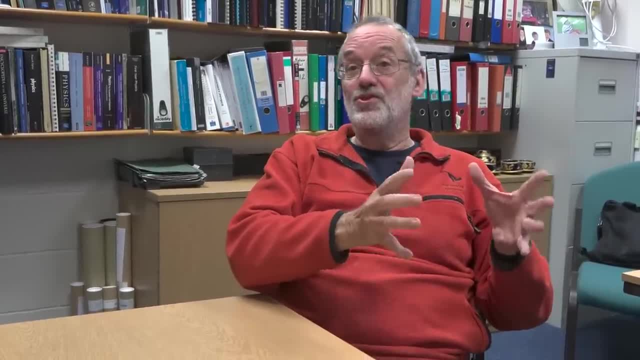 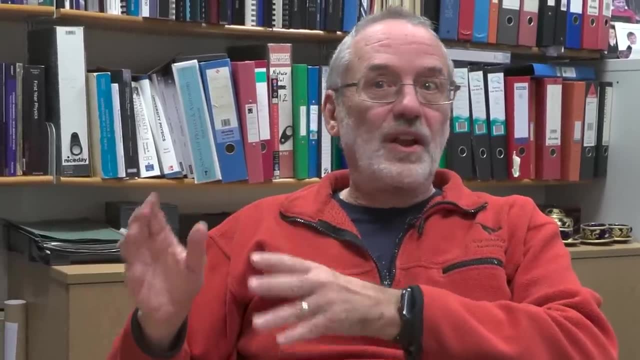 background to it. There are lots of other people whose contributions need to be recognized, But on the other hand, it's just really good to be able to celebrate excellent scientists And clearly the three who won are all outstanding experimental scientists And it's great that they were able to. 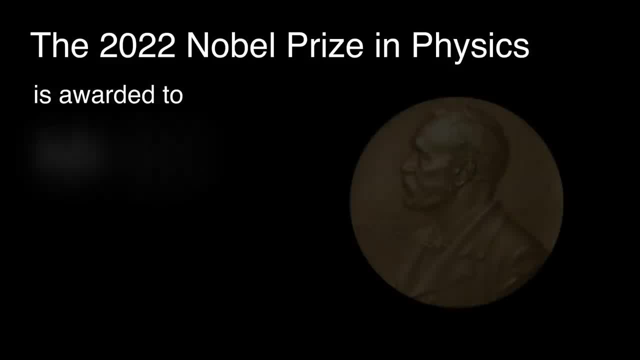 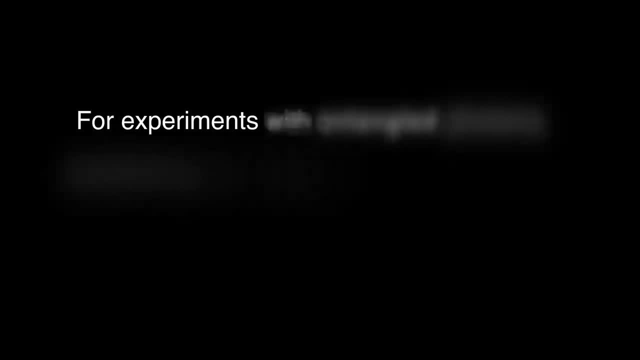 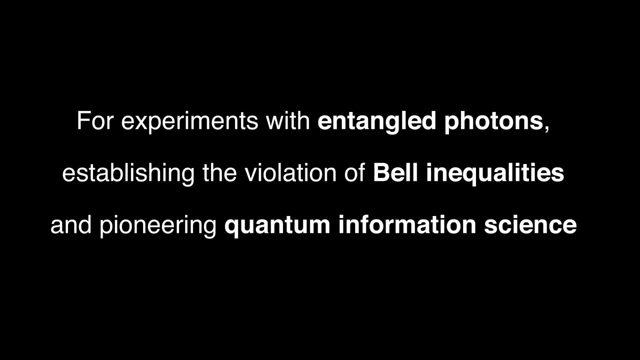 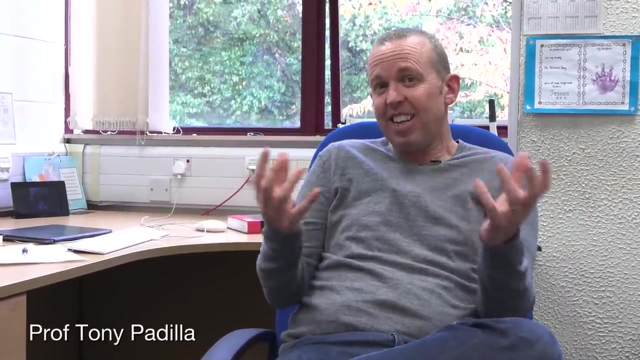 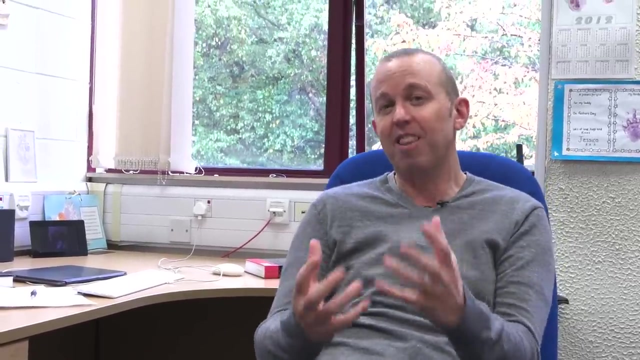 be awarded the prize in this way. My feeling about this Nobel Prize is that it's a real victory for the idea that the universe is. nature is probabilistic. That we live in, you know the underlying ingredients of space and time and the fabric of our universe is fundamentally probabilistic. That's what it comes down to, And 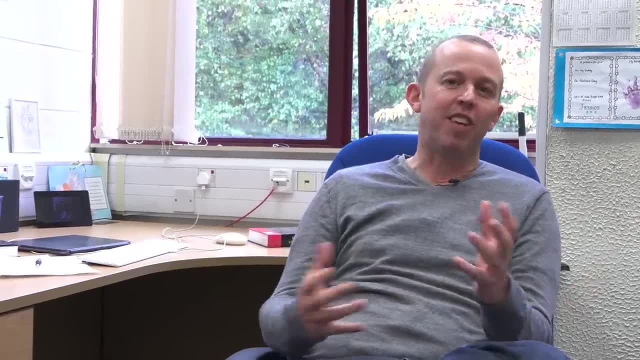 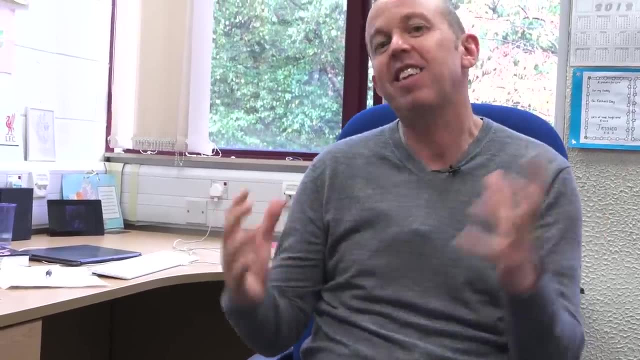 that's what quantum mechanics tells us And that we don't need to have all this other, you know, extra ingredients to try to strong arm our sort of prejudice that somehow everything needs to be deterministic. But no, it's actually probabilistic. 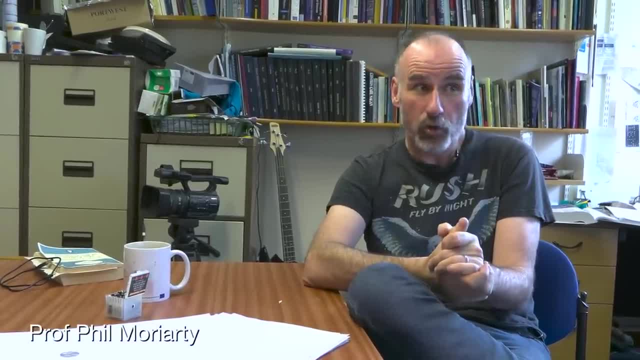 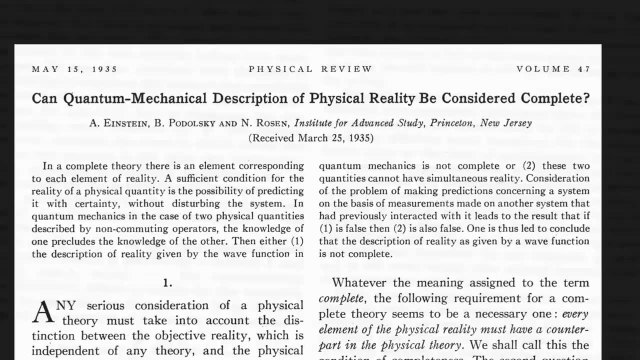 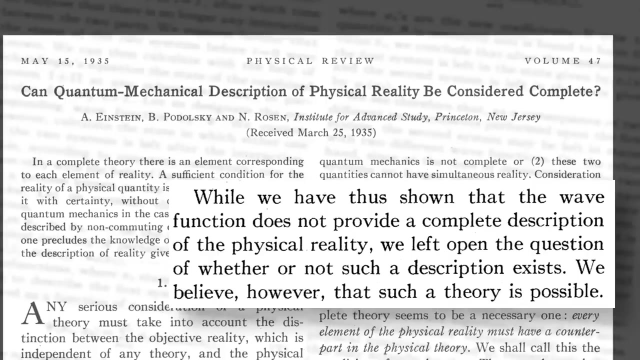 This year's Nobel Prize winners showed that quantum mechanics is right, Contrary to Einstein and his colleagues who published a very famous paper back in the 30s called the EPR paper- Einstein, Poldosky and Rosen- that claimed that, well, there's something missing from quantum. 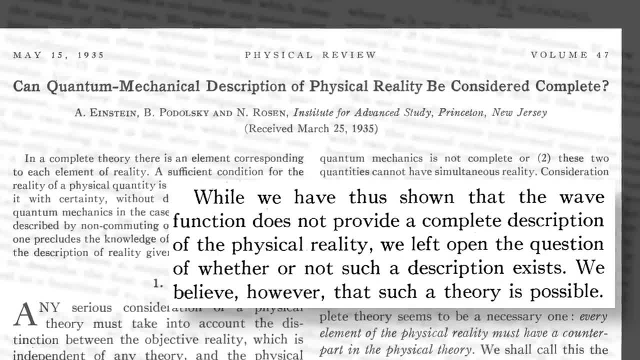 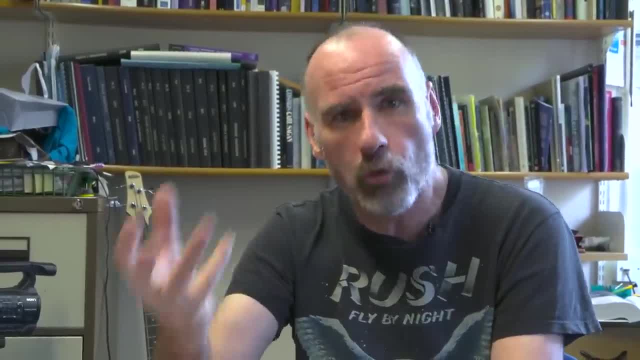 mechanics. It doesn't quite grasp the nature of reality. What this year's Nobel Prize winners have shown is that well, no, I know you're going to hate this and I know it's really uncomfortable and I know it's really unsettling, but quantum mechanics does get the nature of reality. What I'm most happy about is 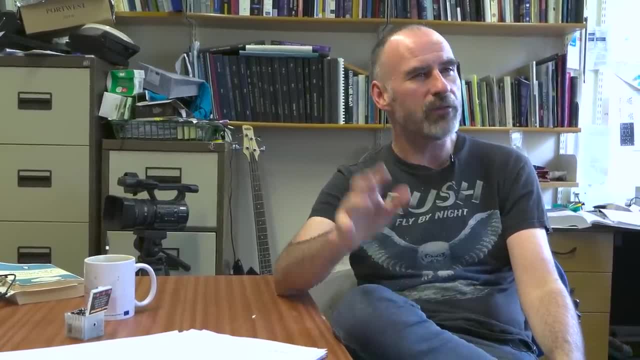 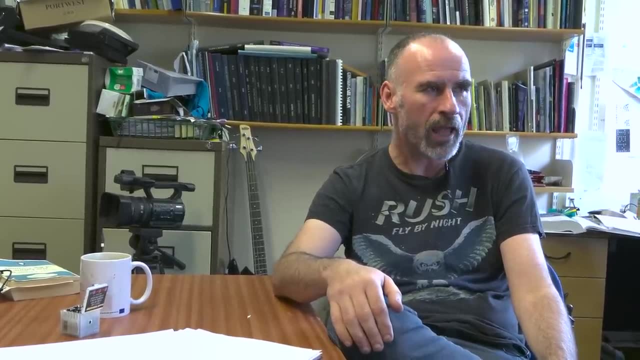 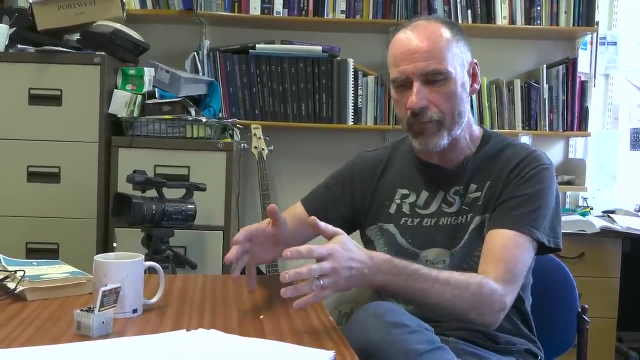 the fact that they've indicated this really famous physicist, a guy called John Stuart Bell, born in Belfast, Northern Irish physicist, And he was the first to say: well, if you do this type of experiment, you make this type of measurements and you look for these correlations. 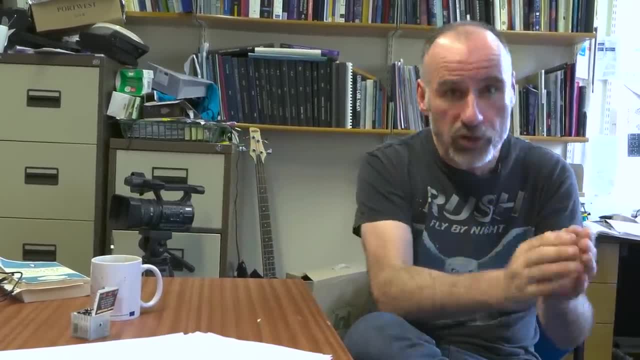 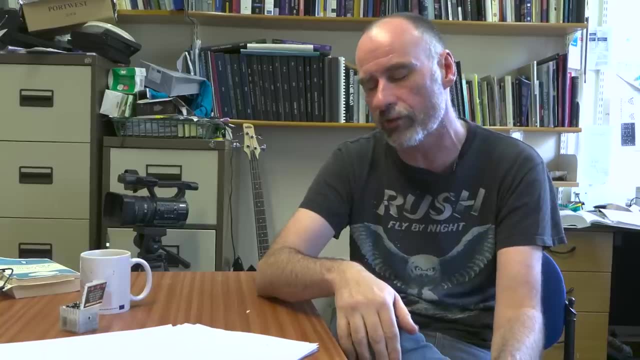 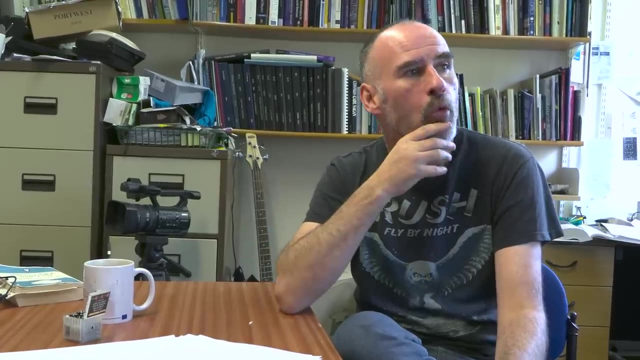 and you think about the statistics, then there is a way of distinguishing between the quantum mechanical view and the view put forward by Einstein- And I know that she was sceptical about quantum mechanics- And it was Bell's- what's called Bell's inequality was described. 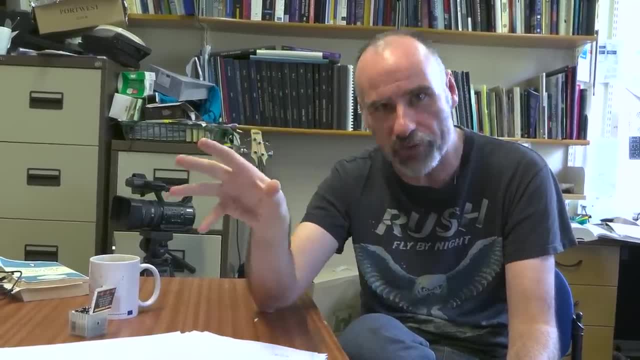 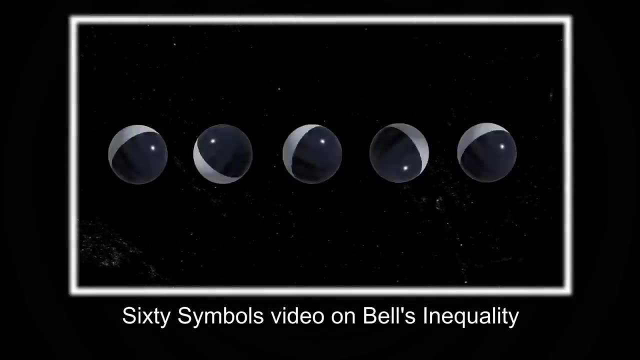 has been described as the most profound discovery in all of science. It's that important because it's telling us about the nature of reality. Very coincidentally, we talk about spooky action at a distance, but on the day of the Nobel Prize it was the day of the Nobel Prize And it was the 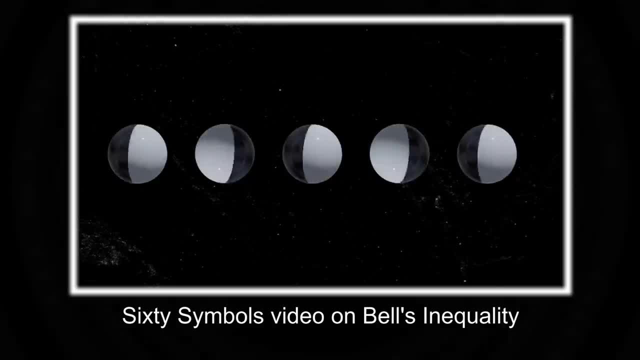 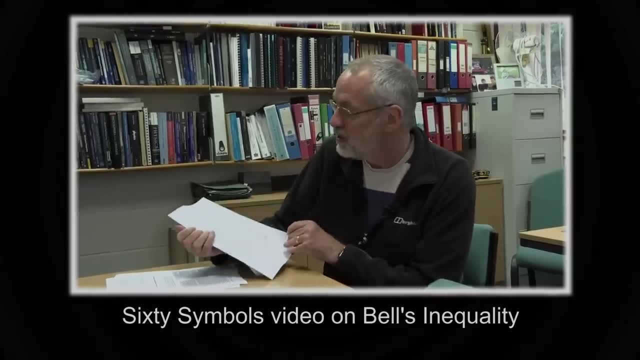 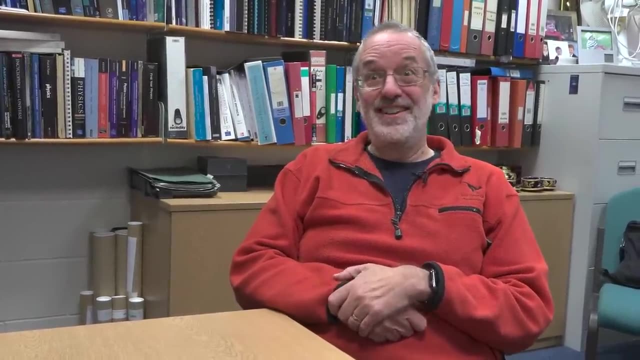 day that the Nobel Prize was awarded, 60 symbols uploaded a video by Mike on the EPR paradox, as it's called, Bell's inequality and just what it's all about. I'd love to be able to claim it's because I had a spy in the Nobel organisation who tipped us off, but actually we didn't. It's a. 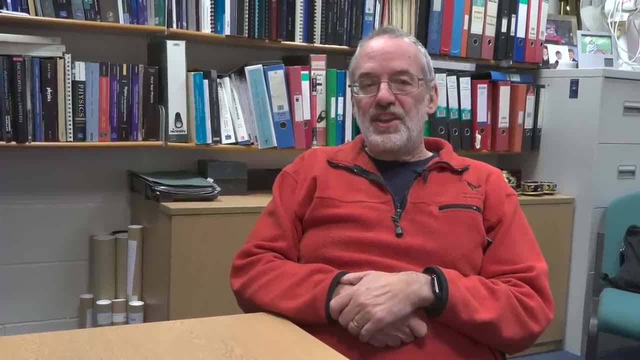 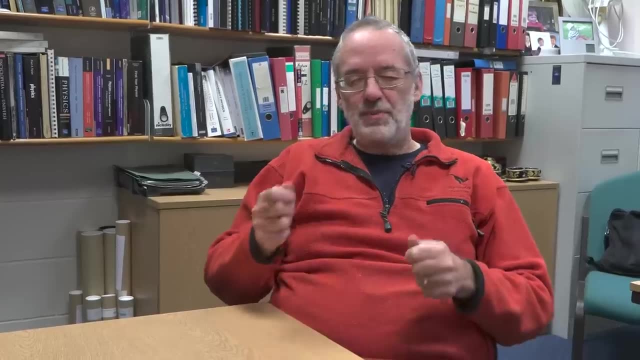 complete coincidence And actually I suspect the reason it's taken us this long to get around to doing a video on Bell's theorem is it's really hard to understand. I mean, it's one of those things. I read the paper and I kind of scratch my head and I 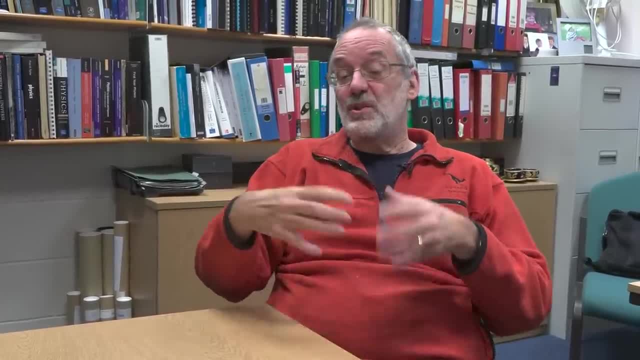 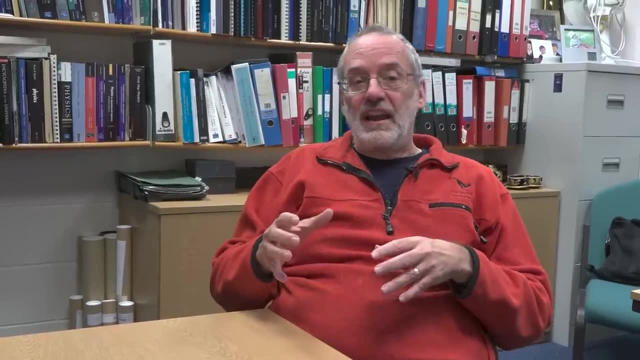 I really focus on it hard. It's a hard bit of physics because it's actually quite a complicated story that goes into the theory. But finally I kind of got my head around it enough to make this video about it a few weeks ago, And so it was. the video was scheduled for release on the. 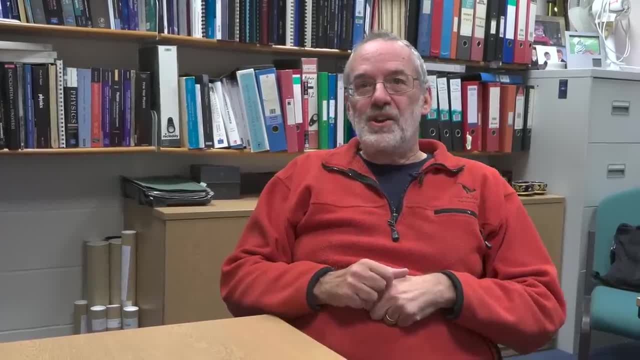 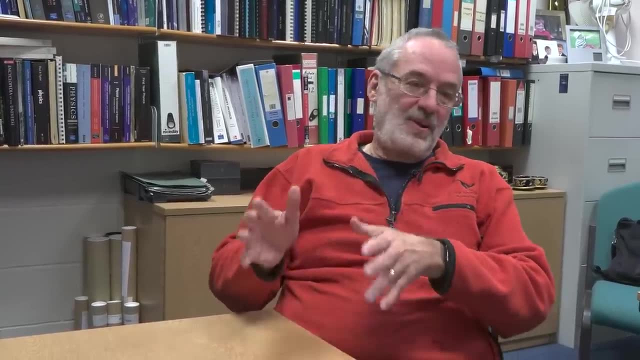 day of the Nobel Prize, by a complete coincidence, And so we were able to look fairly psychic in coming up with this video that came out, you know, within an hour of the Nobel Prize being announced, we had a video out on the physics behind the Nobel Prize. This whole thing is all. 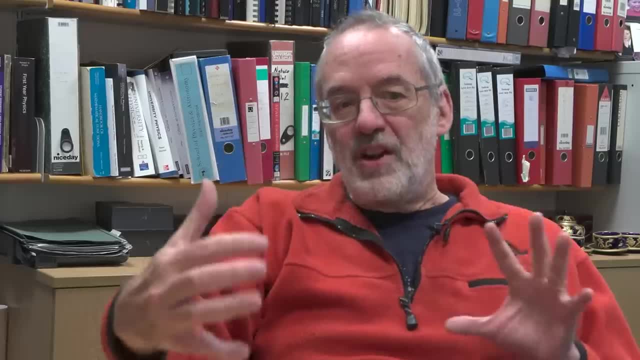 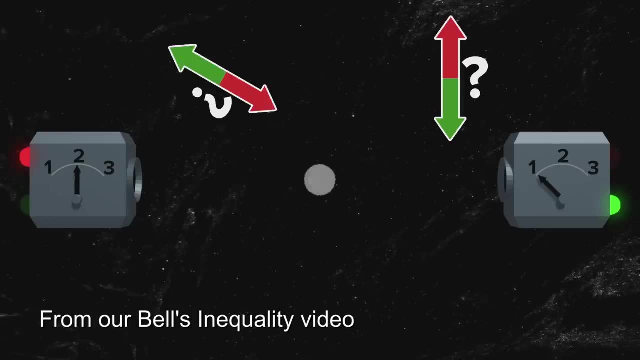 at a distance- as Einstein described it- of things being able to apparently being in contact with each other when they're too far apart for information to pass from one to the other. We kind of did the same thing. We were able to produce a video faster than the information could be brought together to. 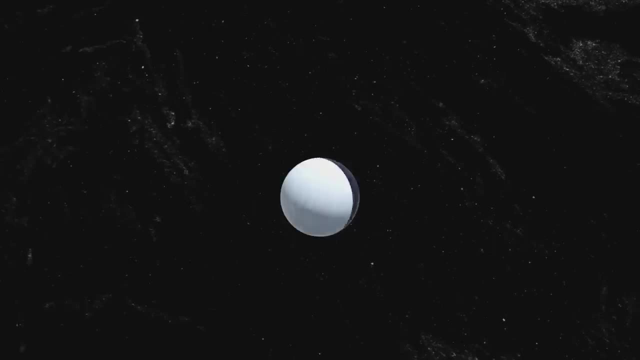 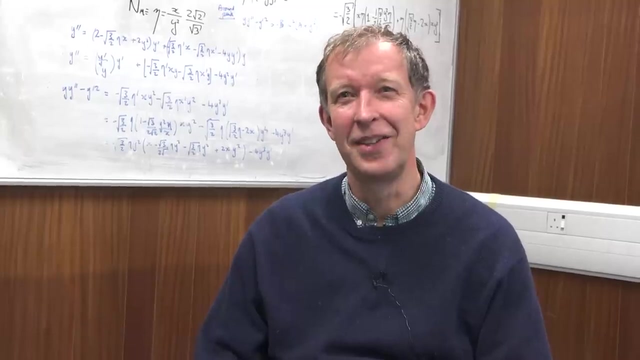 produce such a video, But it's only because we'd actually coincidentally done it a week or so beforehand. It's gone to John Clodier, Alan Aspect and Anton Zellinger. These guys took seriously some original ideas of Einstein Rosen. 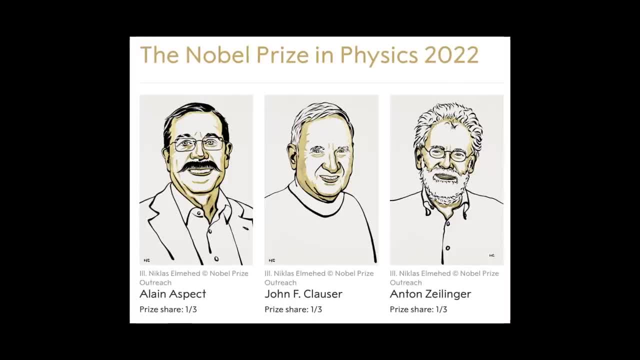 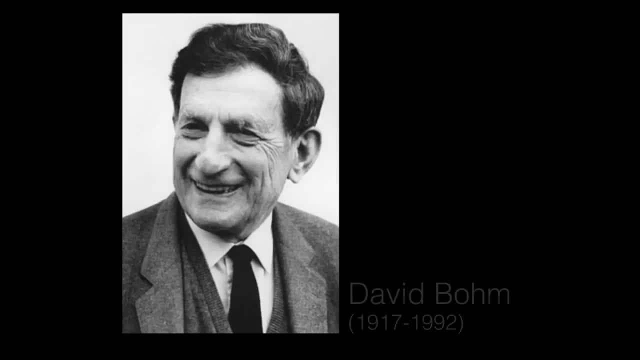 and Podolsky, who were worried about interpreting quantum mechanics, interpreting some of the results of quantum mechanics. that then fed into people like David Bohm, who sort of took their concerns seriously and tried to come up with a kind of alternative way of understanding quantum. 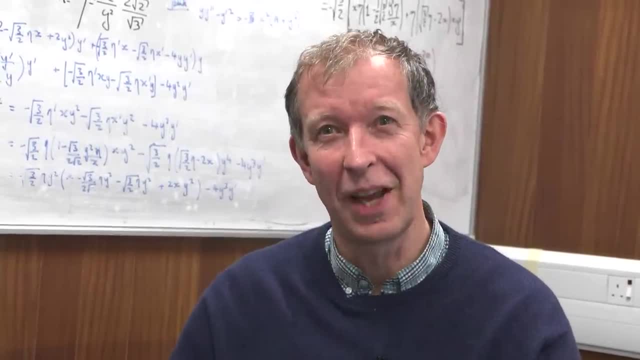 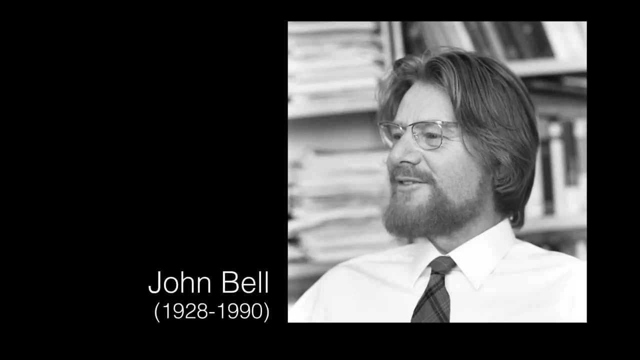 mechanics, which would reconcile some of the issues that Einstein was facing. that then fed on to John Bell, who in turn realized he could discriminate between the ideas of Bohm and then the original ideas of quantum mechanics, and came up with this beautiful mathematical formula, which: 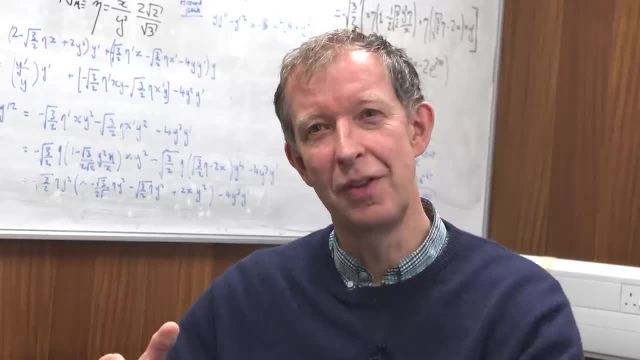 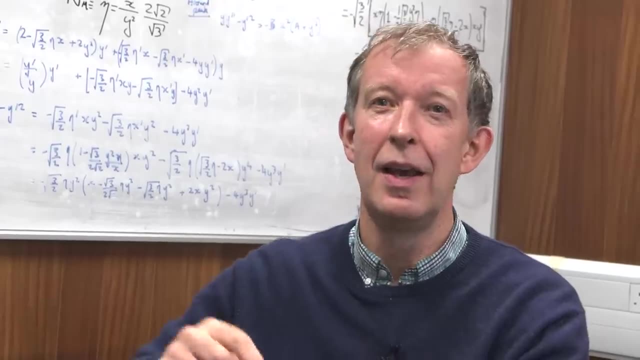 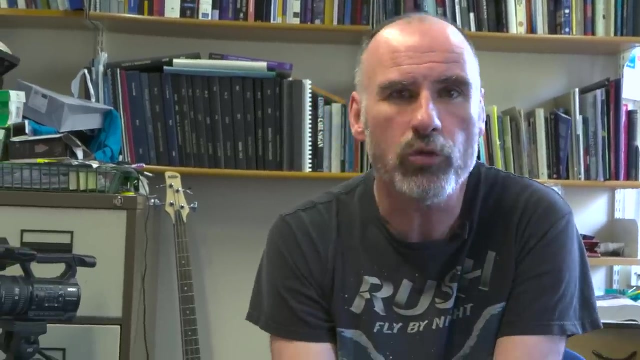 ended up with this bound which, if it was violated, meant that Bohm's what were called hidden variable theories- local hidden variable theories- couldn't be right, And whereas you'd expect quantum mechanics to violate it. The frustrating aspect of this is that they don't award the Nobel Prize. 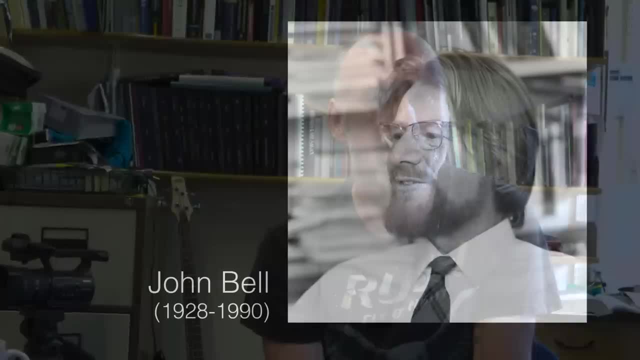 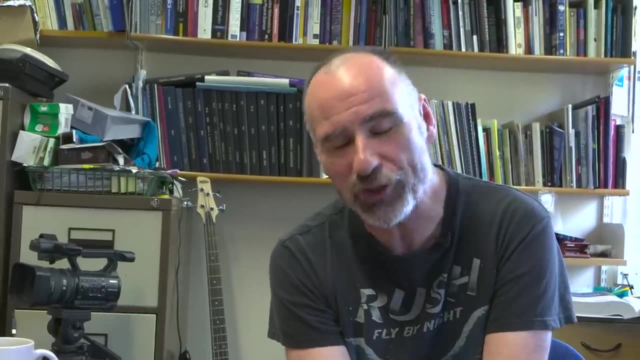 posthumously, So in the year that Bell died, which was 1990, apparently he would go on to be awarded the Nobel Prize. It's really a massive injustice, given that, you know, his discovery, or his inequality, was described as the most profound discovery in science. It's a real 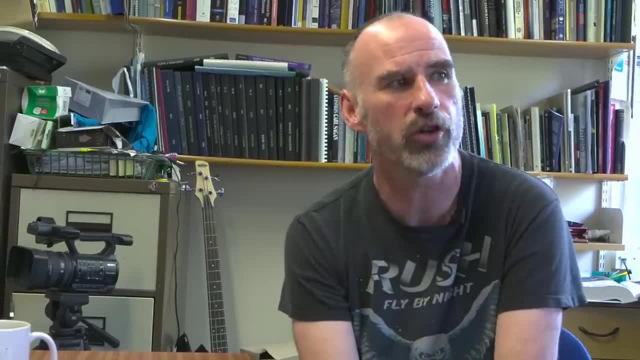 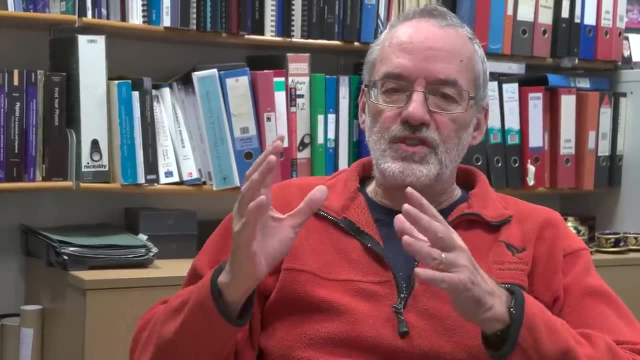 injustice that he didn't get the Nobel Prize, even posthumously. I think we should have a petition- Let's have a petition that he's awarded it posthumously. The point of it was that he showed there was an experiment that would differentiate between whether quantum mechanics was kind of the 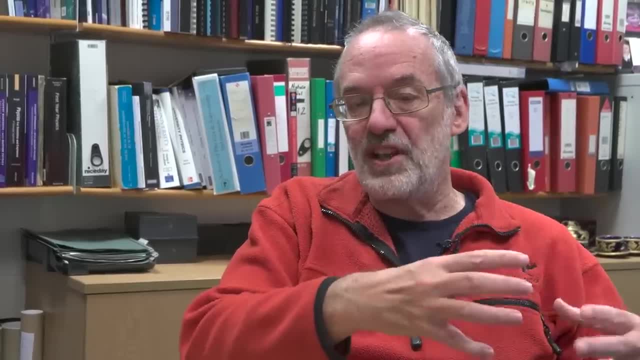 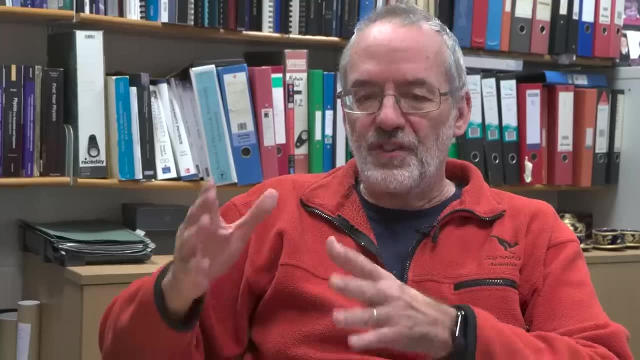 end of the story and the universe was fundamentally probabilistic, or whether there was a bit more physics that we just didn't know yet, Which is a very clever thing to do- to be able to show that you can't. there can't be any more. 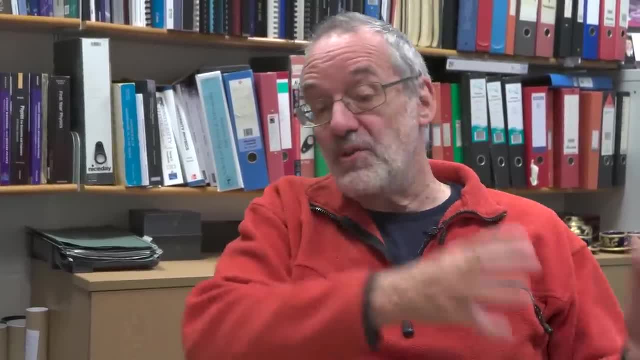 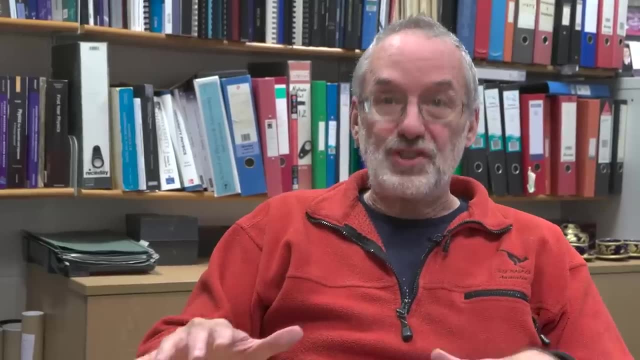 physics is really an impressive thing to do. Anyway, it was a way of distinguishing between these two things, And so this idea that you could distinguish between these two things even in theory was kind of impressive, but it sort of set the scene for an actual experiment that could be. 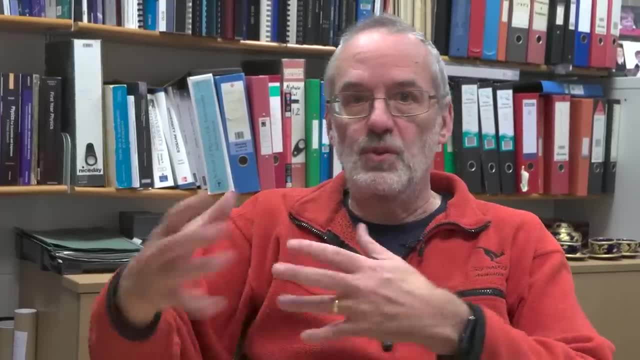 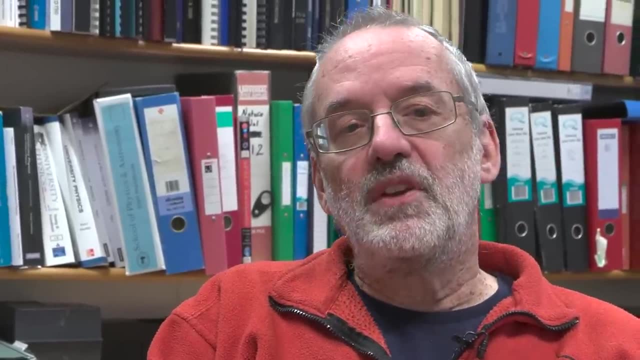 done to tell whether or not quantum mechanics was the full story or whether there was a bit more physics to discover It took a long time. It was one of those very slow burn things, partly because it was a hard experiment to do And partly because it wasn't terribly respectable to think about the fundamentals of quantum. 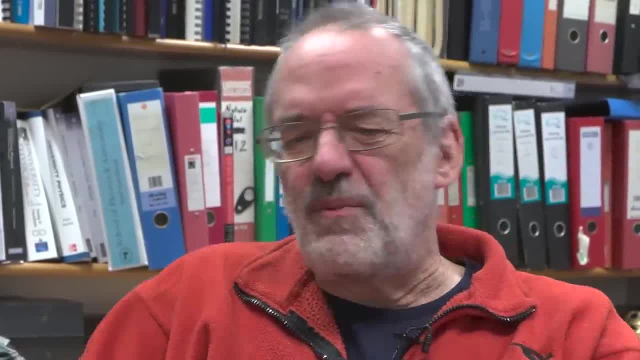 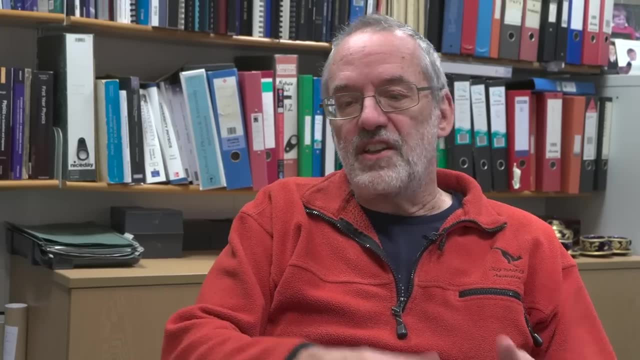 mechanics, It was somehow. it was just. you know, you should be getting on and doing something rather than actually messing around thinking about sort of. it was almost a philosophical argument rather than a physics argument. Of course, the irony is that at the end of it, you know our understanding. 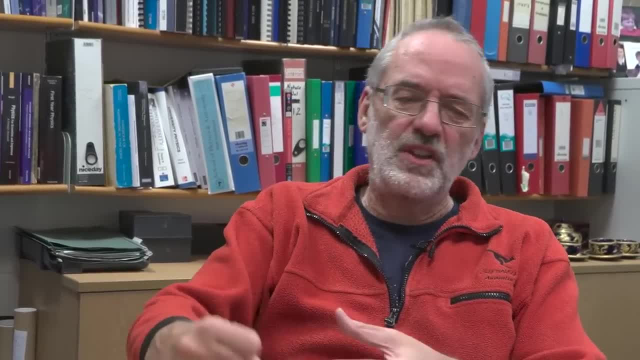 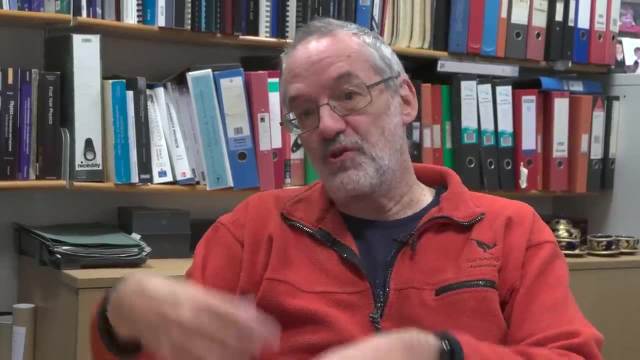 of all the processes involved in quantum entanglement and all the stuff that goes into. it is the basis of a whole load of new physics, a whole load of new technology about quantum computing and cryptography and all sorts of stuff. But anyway, there was a relatively 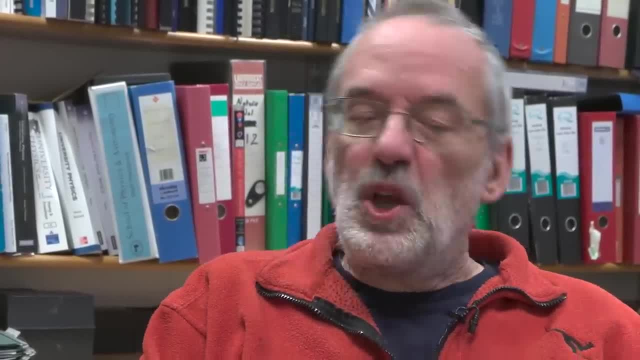 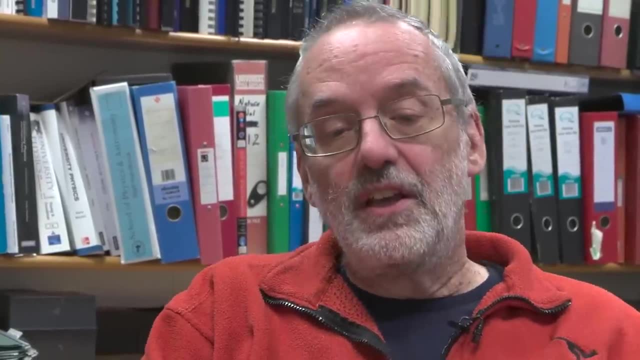 smallish number of people who were working on these experiments, who, over time, did a series of experiments to try and show whether the theory that Bell had put together held up or not. And each time you do an experiment, you know you do the experiment, you say: well, that almost shows. 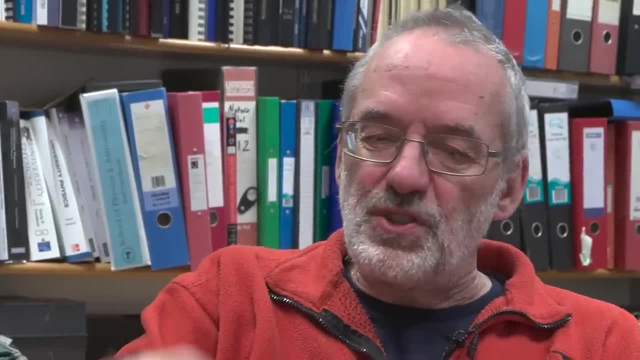 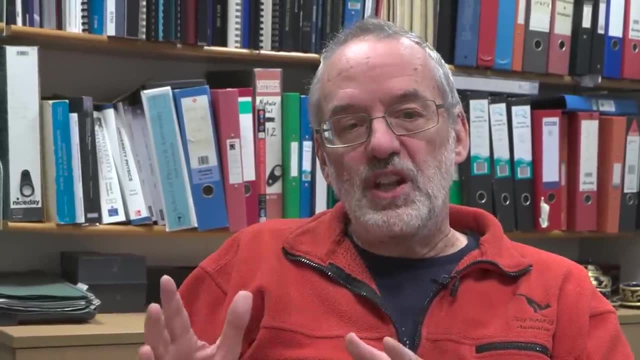 it. but there's this little loophole here, And so there was this series of experiments which successively closed these loopholes off until eventually they really have pretty much been able to show that this Bell's inequality, this Bell's theorem, shows that quantum mechanics is the end. 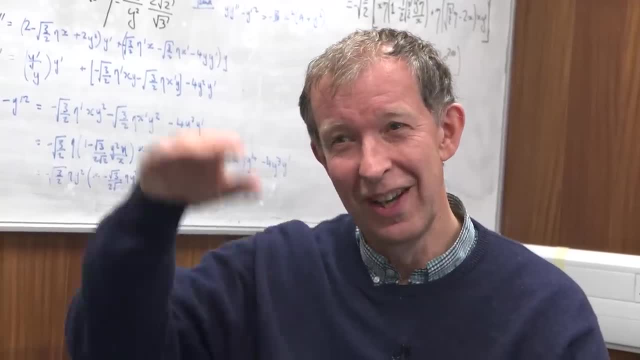 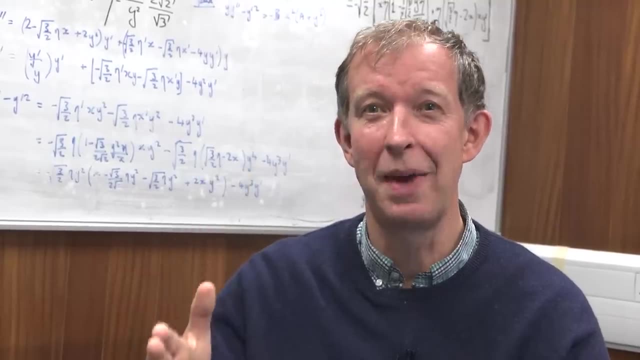 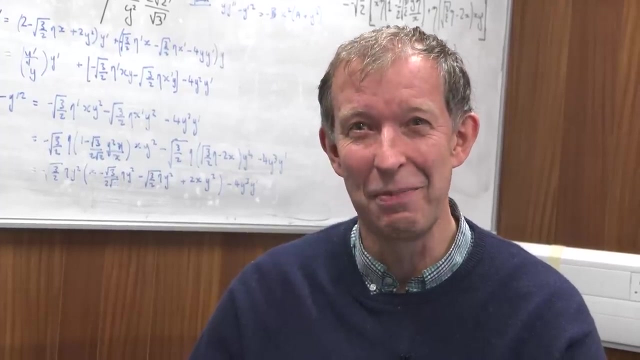 of the story. What these three people have done in this sort of over a series of experiments since the 1960s have basically shown that this bound is violated And therefore quantum mechanics is looking as if it's in a really healthy position and the alternatives like hidden. 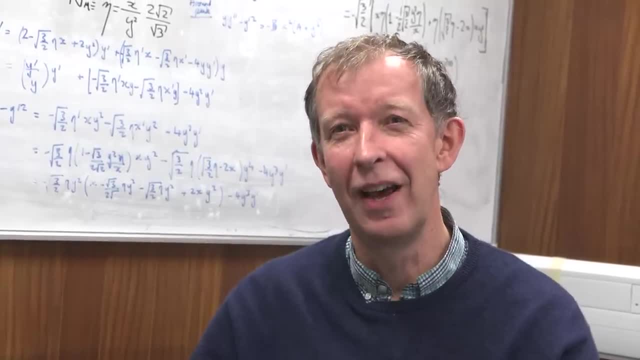 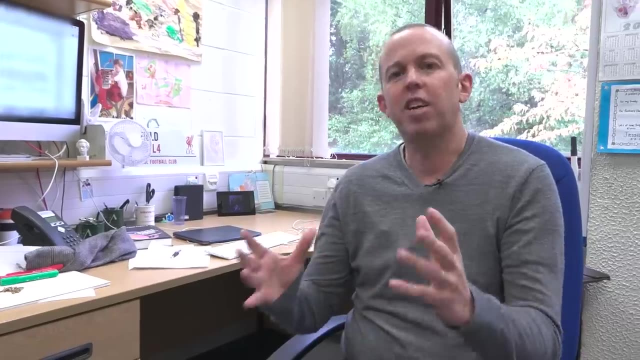 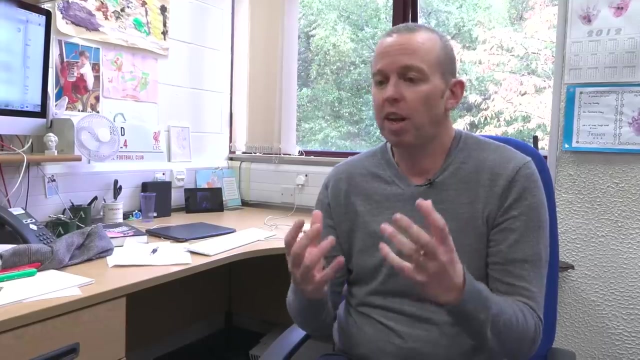 variable theories, at least local hidden variable theories, are in a struggling to explain these and in fact probably can be ruled out. You have an experiment at a quantum level that really things come down to probabilities. Now you know, I can think about, you know, tossing a coin and it has a probability that 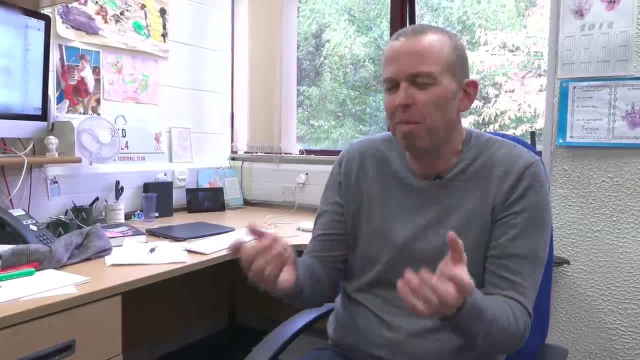 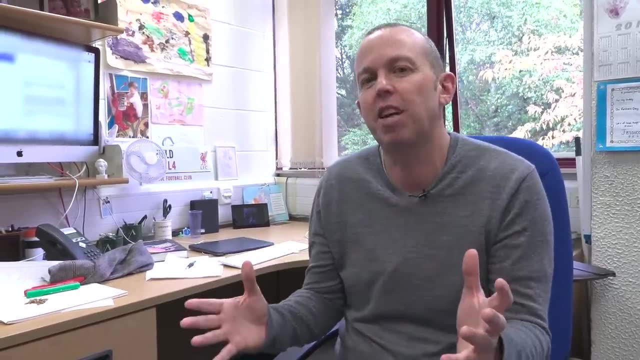 goes heads or it goes tails, But somehow that's kind of a bit misleading because it seems like, well, it depends on how I flick it, you know, and so on and so forth. So ultimately you might think it's actually deterministic, But on a quantum level, you know, there are genuine experiments. that you can do where you really see that there's, and this is what we're talking about. you know, there are experiments that you can do where you really see that there's, and this is what we're talking about. you know, there are experiments that you can do where you really see that there's. 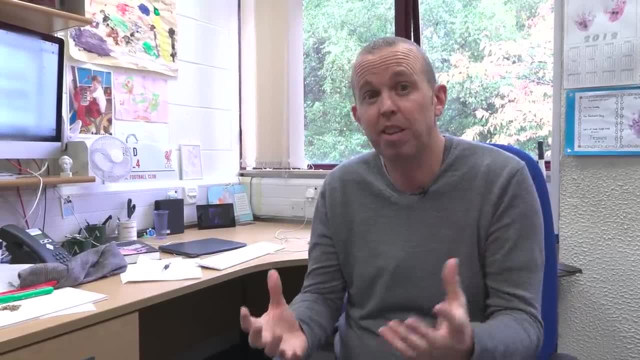 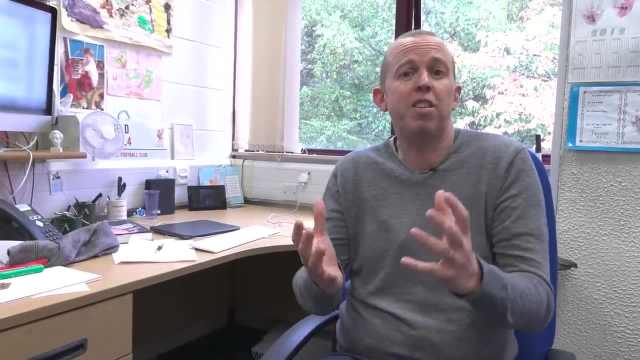 what's related to this Nobel Prize, that really the nature is probabilistic, that you can have a, say, an electron, And you know when you you might want to measure its spin, and whether you measure the spin as being sort of spin up or spin down. you know it's a truly probabilistic. 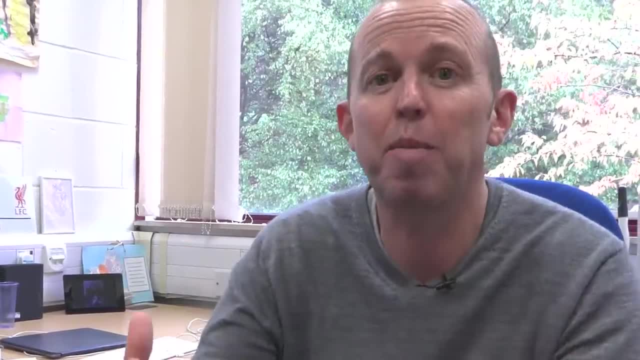 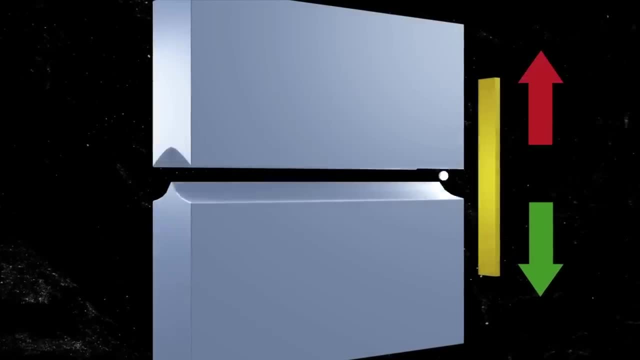 thing. It could be either- and it's in some sense both, And until you perform the measurements it's, you don't know. And this is just how nature works. on a sort of the most fundamental level. It really is truly probabilistic. Some people don't really struggle with that. 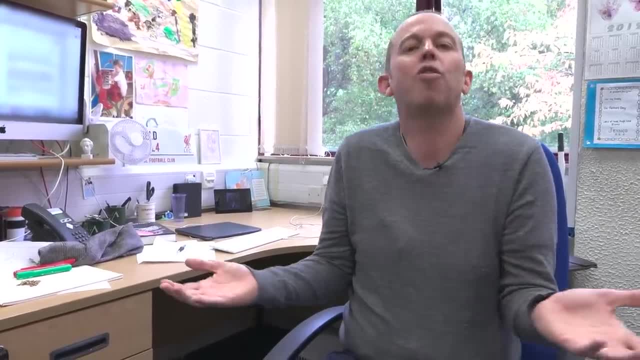 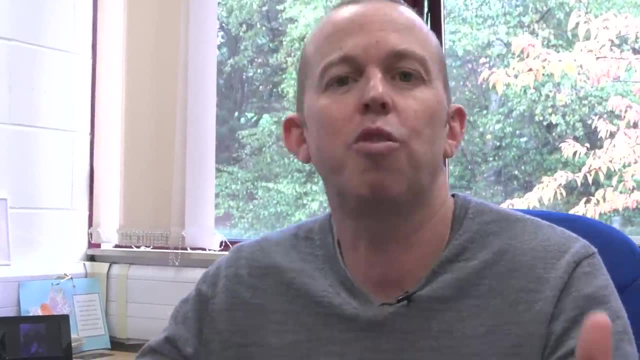 but I don't really see why. I mean, I always think of like a horse race and there are probabilities beforehand for one horse winning over another, and that's fine, And then the horse, a particular horse, wins the race and nobody freaks out, right? That's okay. It's just probabilistic, right? But